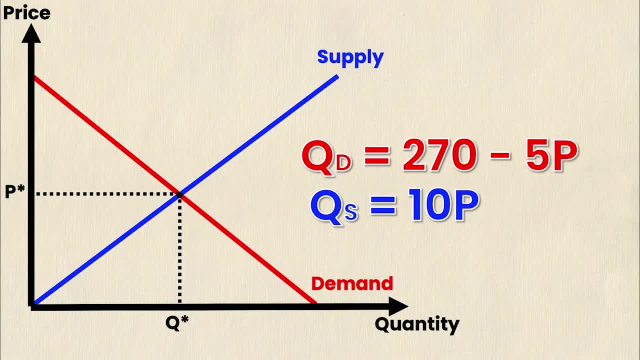 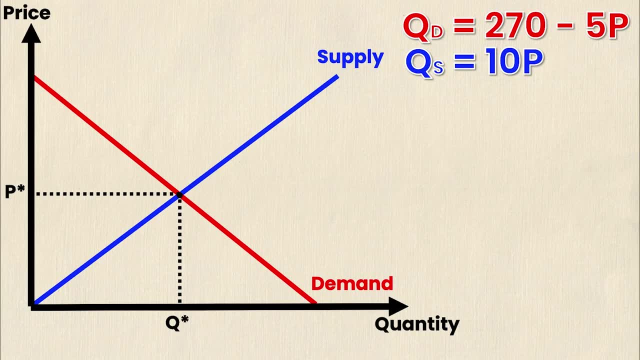 is equal to 10p. So now that we have our demand and supply equation, we're going to take note of them and we're going to use them to calculate four key points on this generalized supply and demand graph. The first point is where the demand curve intersects the price axes. The second point: 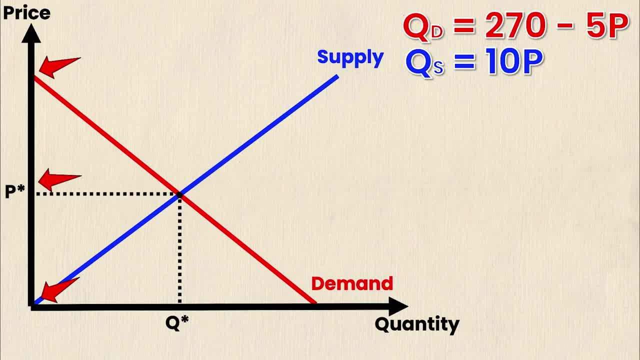 is where the supply and demand graph intersects the price axes. The second point is where the supply curve intersects the price axes, And then we have p star and q star. Once I've calculated those four points, I'll be able to calculate consumer and producer surplus. Let's begin by 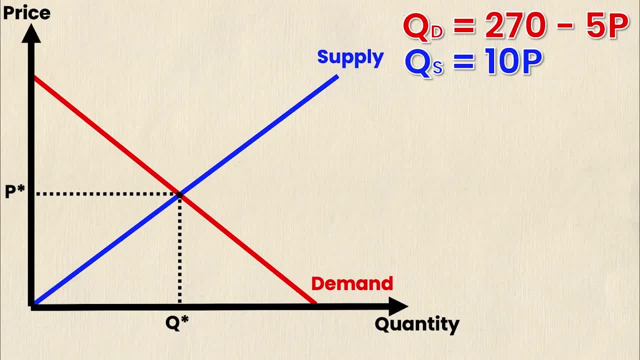 calculating equilibrium. So if you aren't sure how to calculate equilibrium, we'll be doing that in this video. However, if you need extra practice, we have other videos on our channel which are dedicated exclusively to calculating equilibrium, price and quantity. So please take a look at those. 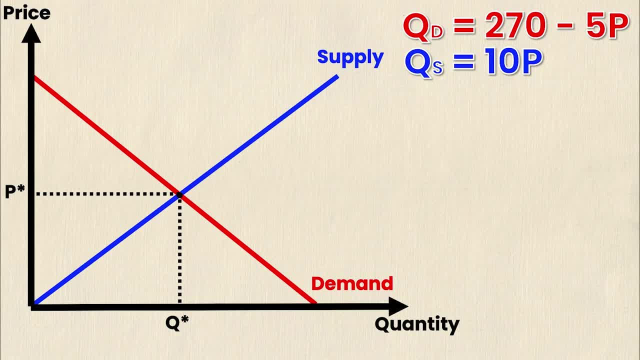 if you find yourself needing more practice. However, as this is a step by step, I'm going to be going over how to do that in this video as well. So, when calculating p star and q star, you simply set the demand equation equal to the supply equation, and that's going to yield us. 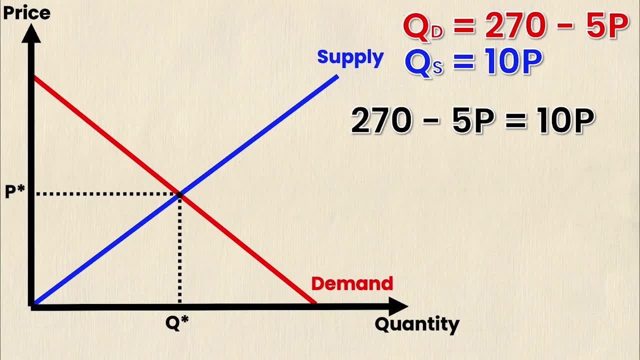 270 minus 5p is equal to 10p. After some simple rearranging, I get 270 is equal to 15p. And then finally, isolating for p, I get p star, or the p value at equilibrium is equal to $18.. Now that I 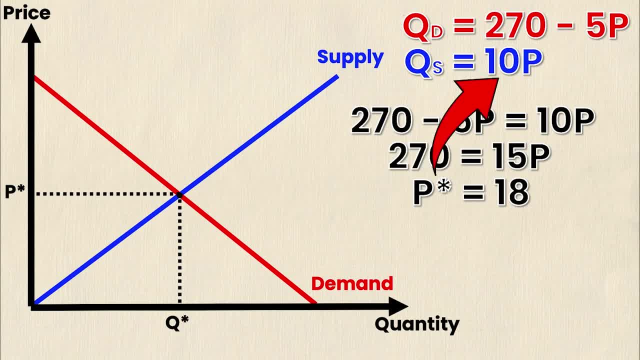 have p star, I can sub it into the quantity demanded or quantity supplied equation. I'm going to use the supply equation because it's significantly easier. However, no matter which one I sub it into, it's going to give me the same value for q. So subbing it into the supply equation. 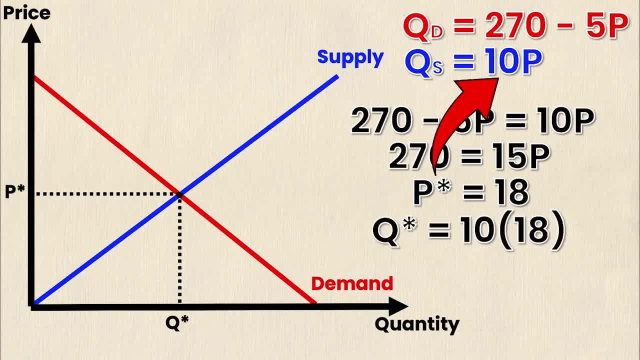 I get q star or q at equilibrium is equal to 10 times our new price, which is 18.. 10 times 18 is 180.. And therefore I now have my q star, which is 180.. p star is 18 and q star is 180.. So let me. 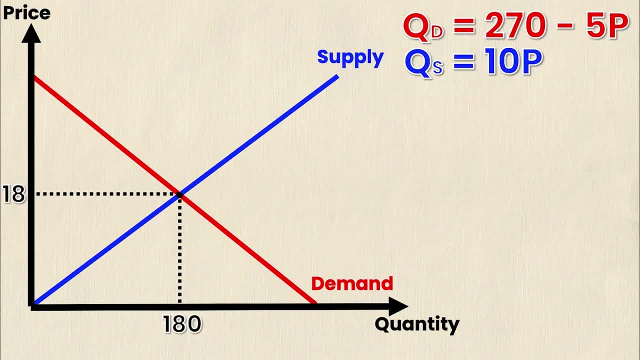 transfer those values onto my graph. Now that they're labeled as p star, I can sub it into the on my graph. instead of q star and p star, I actually have their values. I'm looking for two more points. That is, where the demand curve intersects the price axes and where the supply. 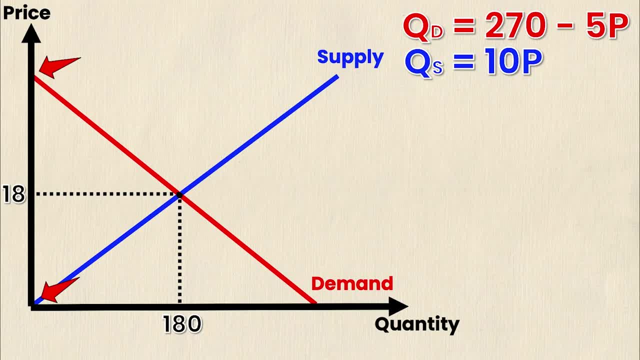 curve intersects the price axes. So these are the last two points. I need to calculate consumer and producer surplus. So how do I do that? again, Well, anywhere along the price axes. we know that the quantity is zero. That is, for a y-intercept, the x value must be zero. So all I need to do for each 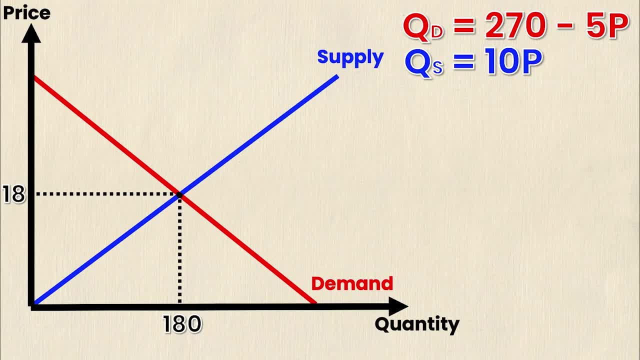 equation is: set quantity equal to zero and solve for that. So I'm going to do that again. So I'm going to do that again for p and that's going to give me my p-intercept or my y-intercept. in this case, Let's start with the demand equation, which will yield us the price intercept for the demand. 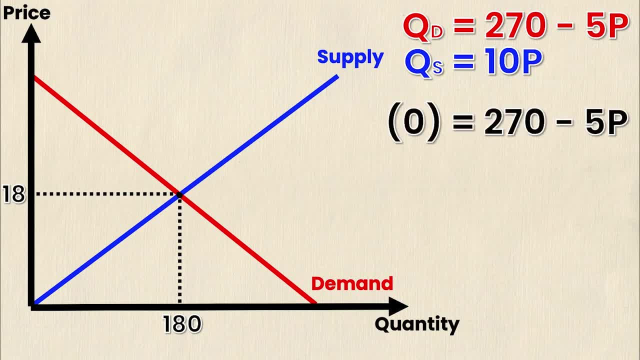 curve. So, subbing in zero for q, I get zero is equal to 270 minus 5p. Rearranging, I get 5p is equal to 270. And then, finally, isolating for p, I get a p value of 54. So that is my p-intercept. 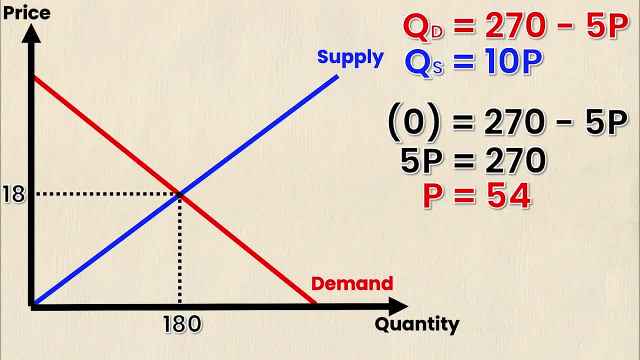 for the demand curve. Doing the same thing for the supply curve, I'm going to do the same thing for the supply equation I get: zero is equal to 10p. Well, this one's even easier- P must be equal to zero as well. Now that I have my p-intercepts for the supply and demand curves, I can now label those. 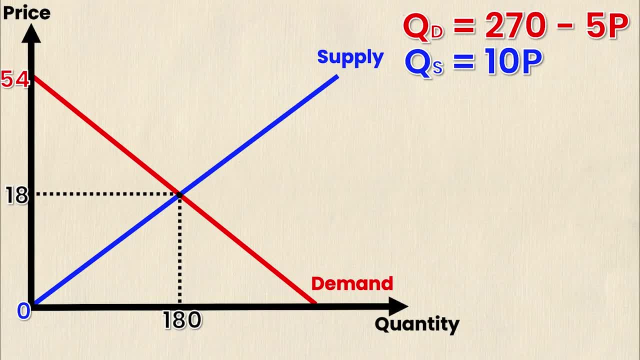 on the graph as well. So, now that everything's labeled, we're onto our final step, and that is actually using these four points to calculate consumer surplus and producer surplus. As for the supply and demand equations, well, now that we've used them to calculate these four values, 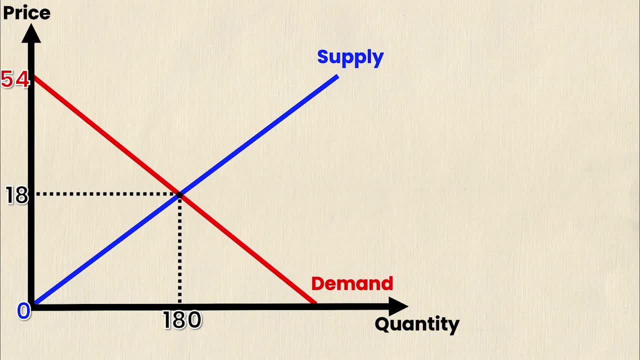 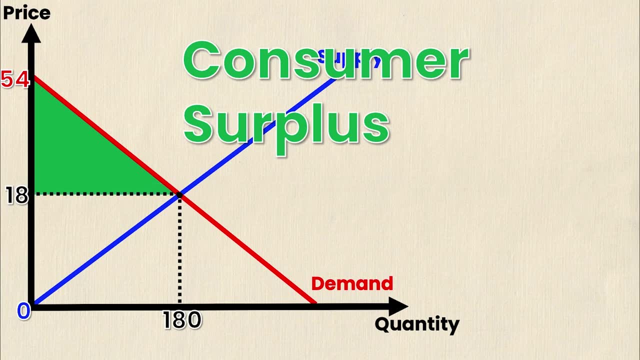 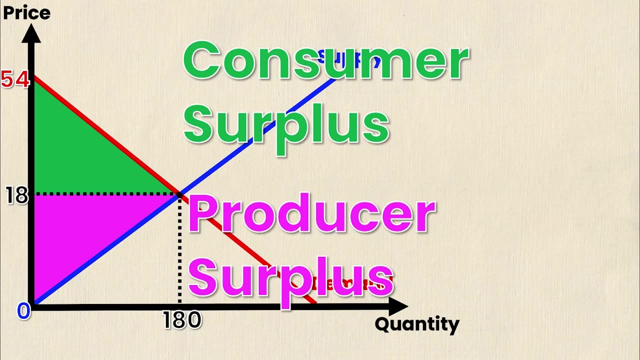 we no longer need them anymore, So let's get rid of them. Now. remember: consumer surplus is the area below the demand curve and above the market price, and producer surplus is the area above the supply curve and below the market price. So all I need to do is calculate the area of these two. 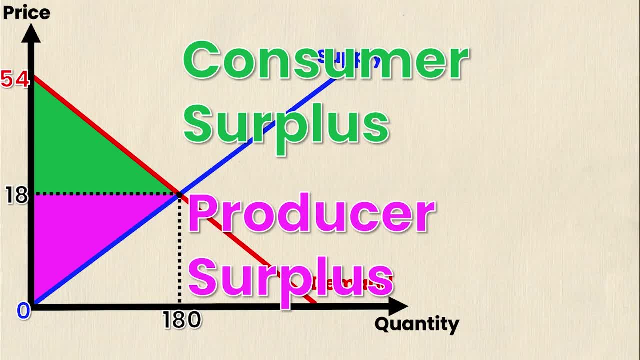 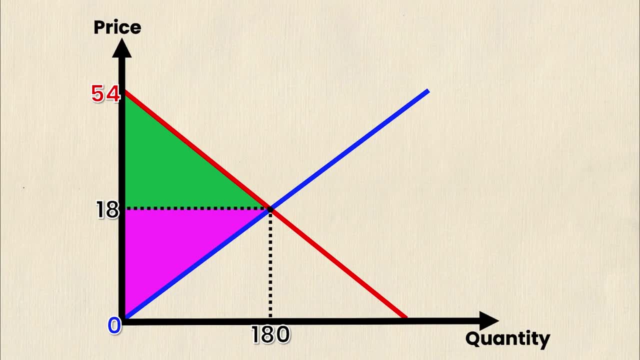 triangles. So let me center out this graph in the middle and we'll start solving. The area of a triangle is simply equal to base times height divided by two. We'll start by calculating consumer surplus For the green triangle. here the base is 180, and the height is 36.. The height in this case is